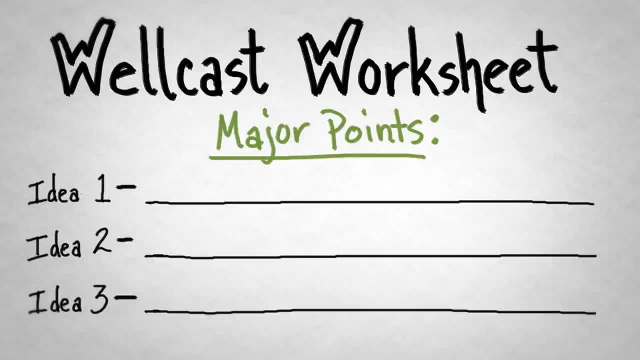 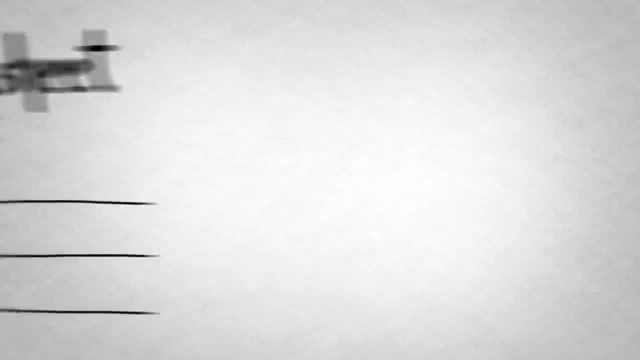 In your Wildcast worksheet, write down the major points that you want to get across to the audience. Get the ideas out of your head and onto the paper. In the next column to the right, start ordering these points in a logical manner. Arguing your point to the audience and wanting them over is like 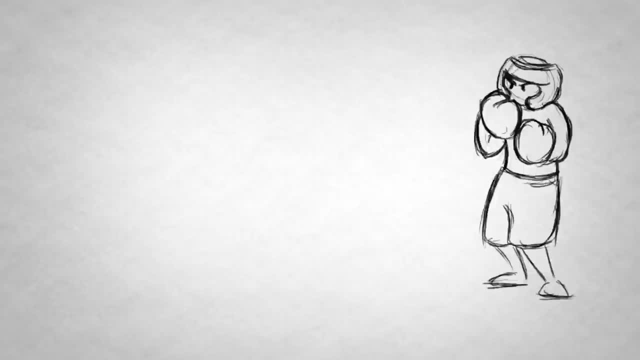 a boxing match. First start with some fancy footwork. A fact or an anecdote that will hook the audience in and get them to pay attention to you. Then throw a couple of swings Supporting evidence for your argument: Stats, personal stories. 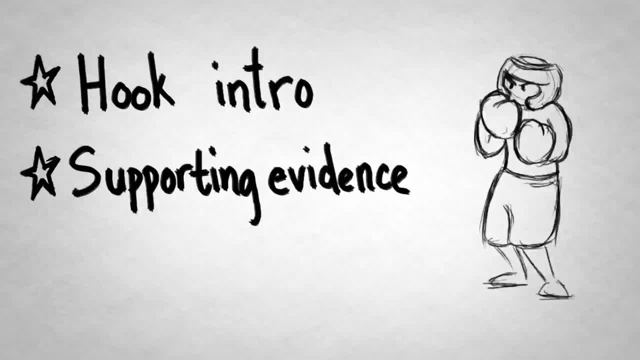 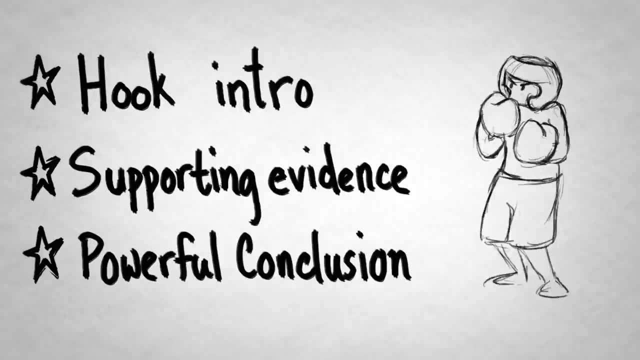 Something that will start to convince the audience that you're taking control. And finally, the knockout, A landing blow of statements that's memorable, convincing and sums up your speech's position Alright. step two: Posture and physicality are key. 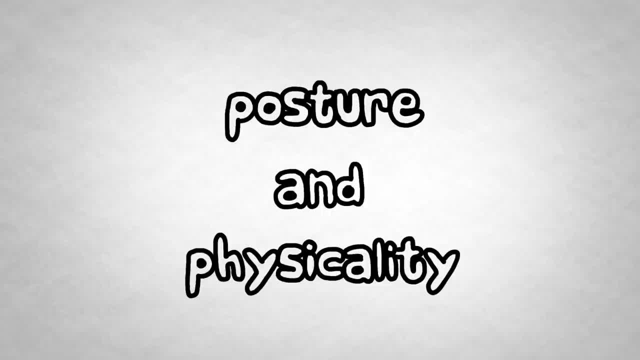 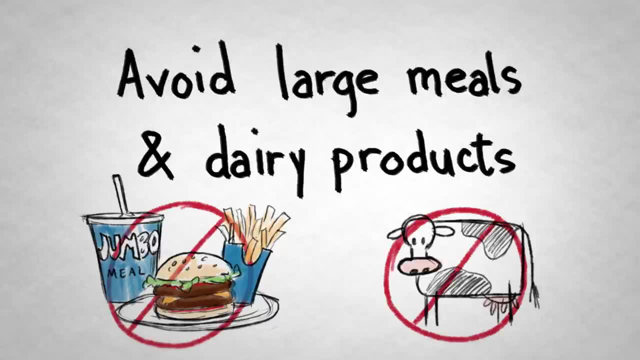 Part of keeping your anxiety at bay while giving your speech is knowing what to do with your body Before your speech. avoid large meals or dairy products, which will make you feel like you need to clear your throat incessantly. Bring a bottle of water on stage if you're allowed. 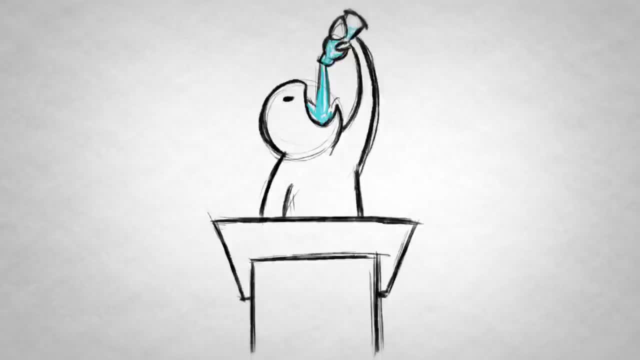 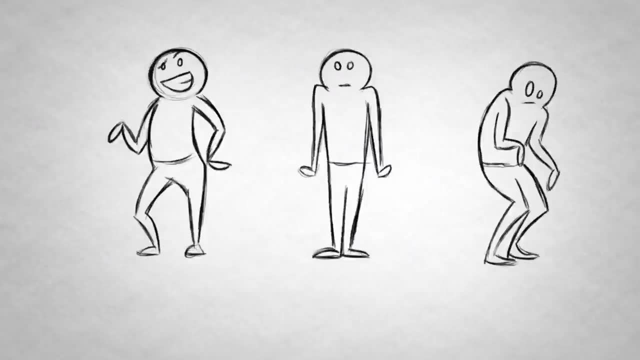 Don't be afraid to take sips throughout your speech. It'll keep your voice natural and it gives you a moment to pause and regain your composure if needed. Stand naturally, Not too stiff or slumped. Good posture will help you breathe and speak easier. 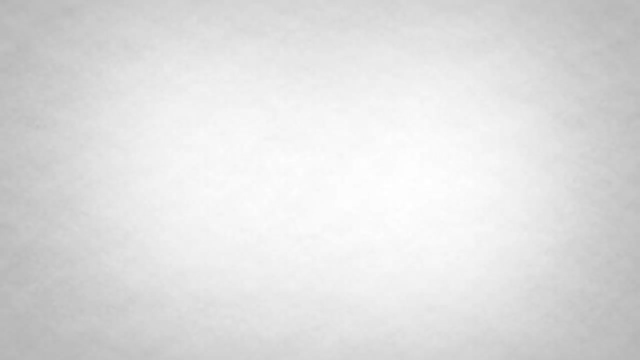 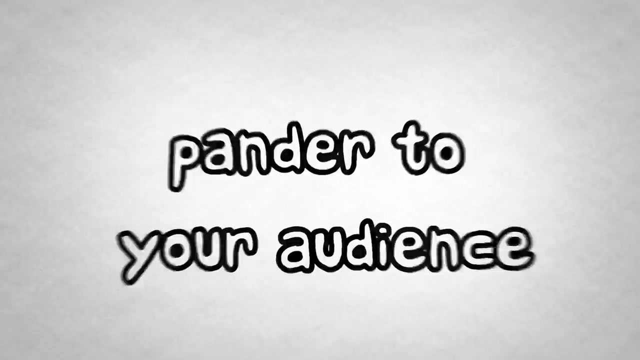 And it'll let your audience know that you're calm and in control. Step three: Panda to your audience. The best public speakers know how to work the room. Don't be completely serious unless the occasion calls for it. Don't read entirely off the cards. 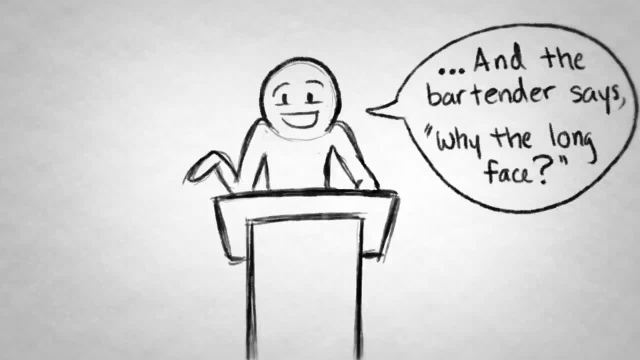 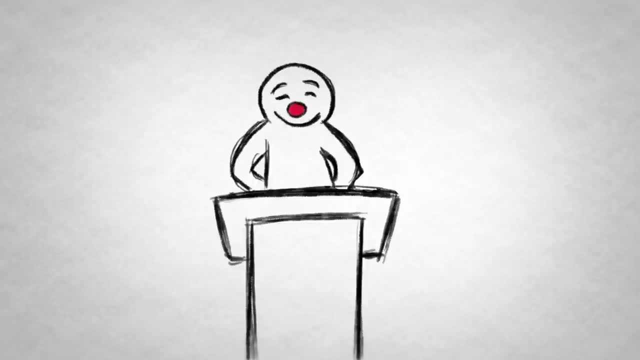 Keep a natural cadence and pace. Throw a joke or a side in- It'll draw in a laugh. If there's a silence, then turn that into a joke. Stay natural, Self-effacing, And the audience will be on your side. 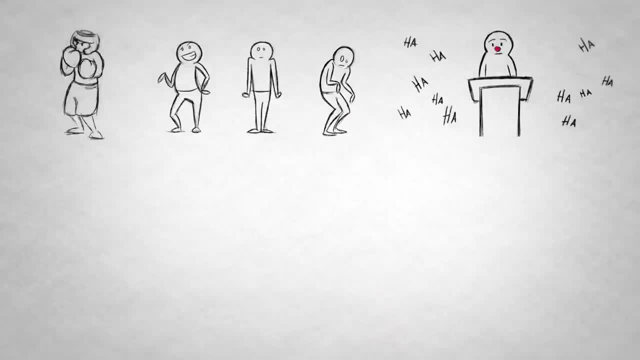 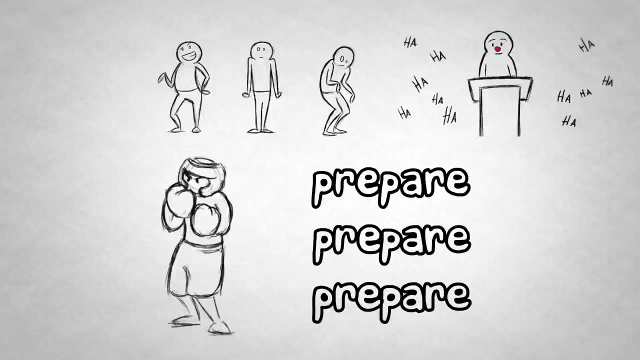 Let's recap: You'd rather face a poisonous reptile than public speak, huh Well, follow the well-cast Triple P checklist. Prepare extensively for your speech, Know your content backwards and forwards And figure out the absolute best way to present it and to win over your audience.